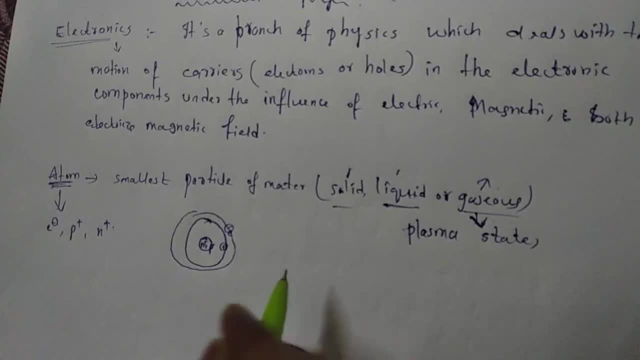 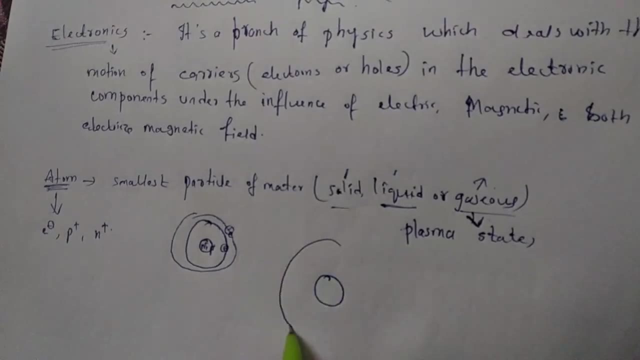 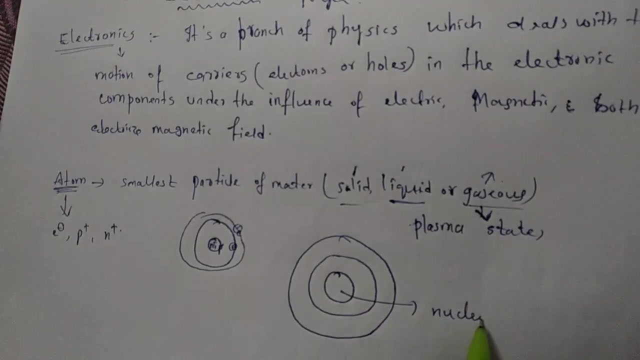 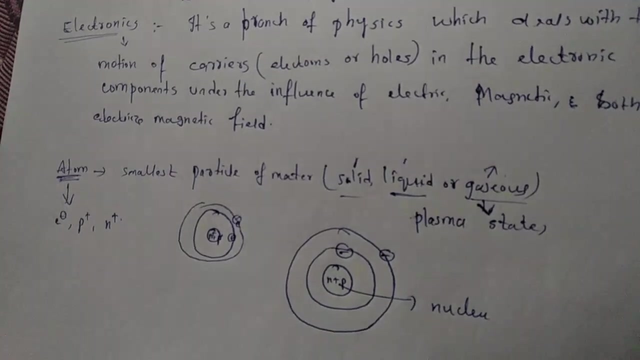 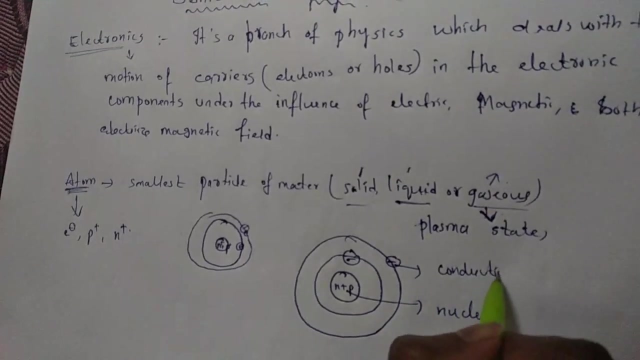 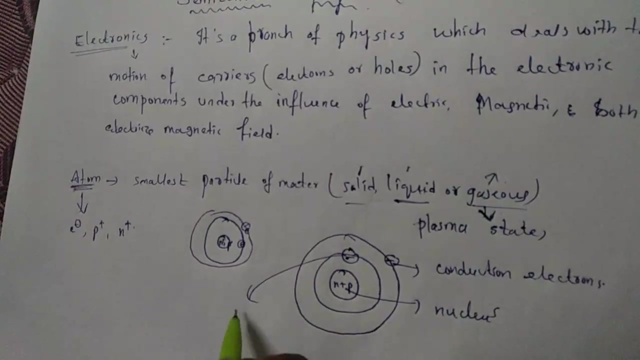 in the outermost orbits there will be electrons which is revolving around the nucleus. this is nucleus. these are the electrons revolving around the nucleus, and the outermost electrons are known as conduction electrons. the electrons that are near to the nucleus are known as valence electrons. 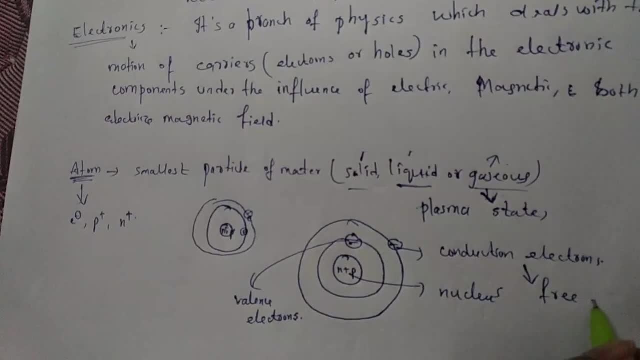 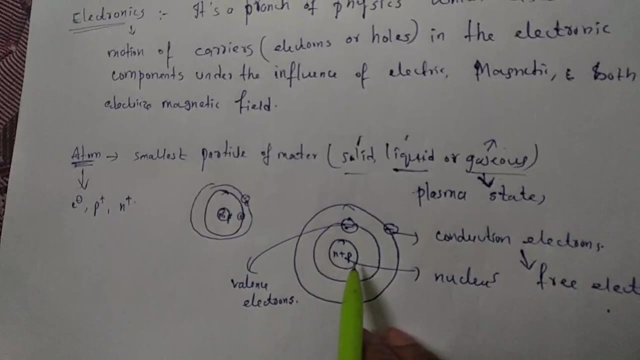 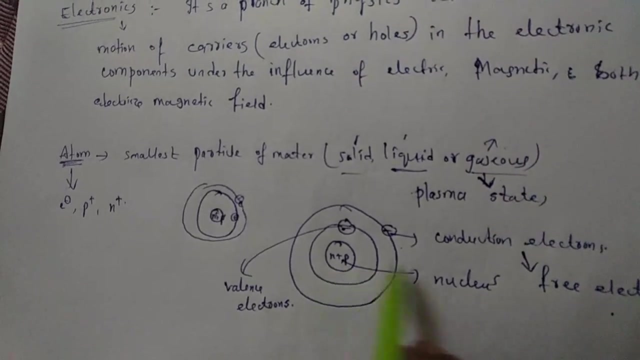 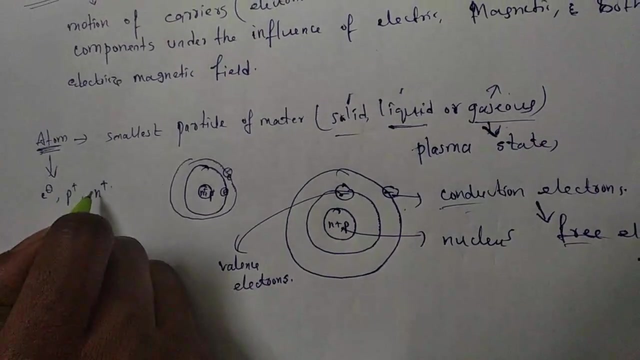 and this conduction electron is also known as free electron. the conduction electron or free electron means the electron which is very far away from the nucleus and has very less force of gravity or attraction due to the nucleus. these are conduction electrons or free electrons. now we'll see the how the electron masses and charges are. 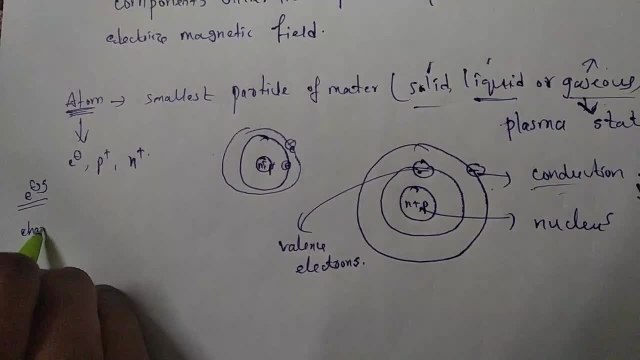 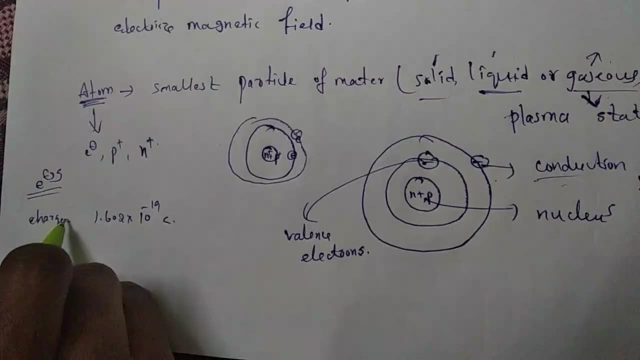 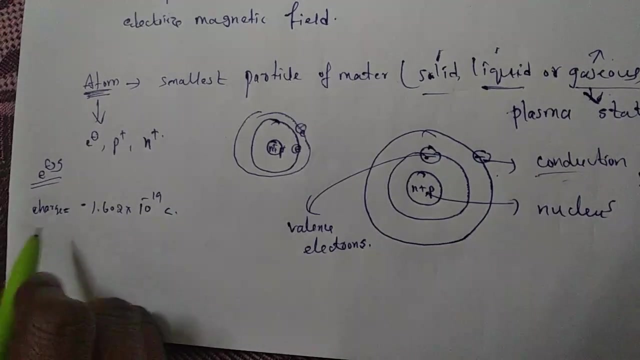 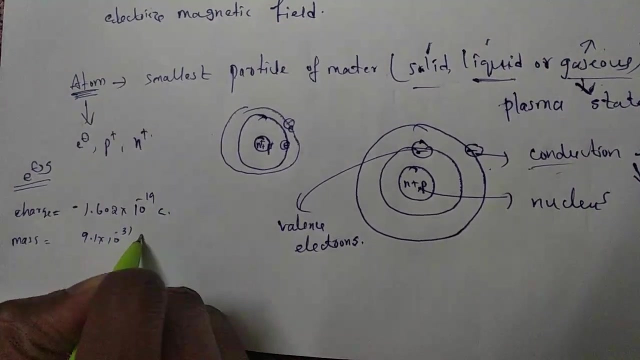 now we'll see the electron mass and charge. charge of electron is 1.6 minus 19 columns, as the charge of electron is negative. so the charge will be minus 1.6, 2 into 10 power minus 19 columns, and the mass is 9.1 into 10 power minus 31 cases. 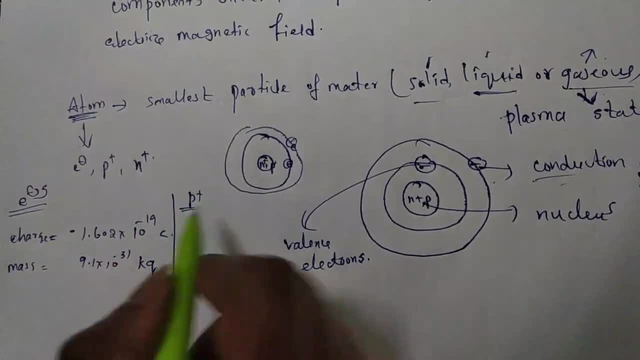 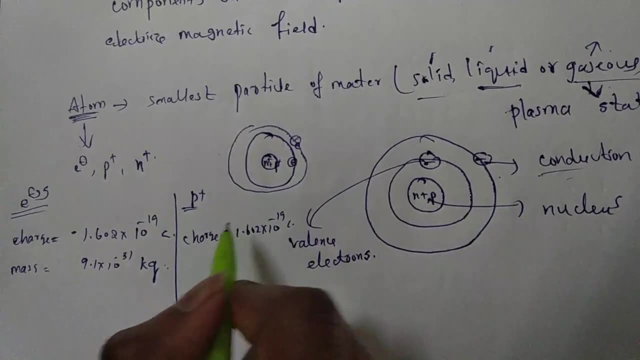 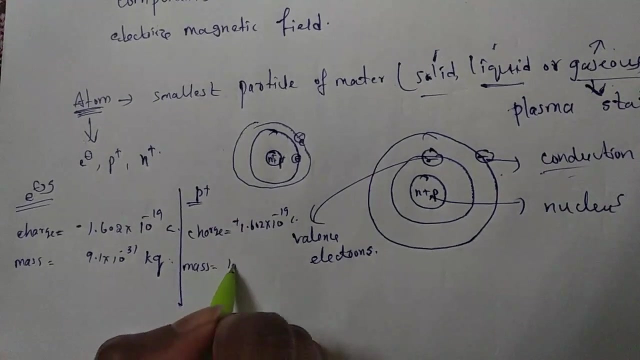 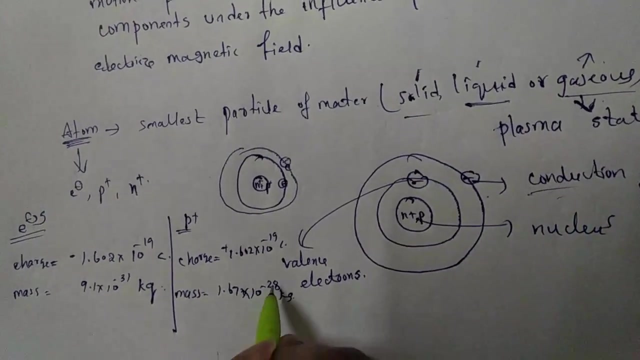 and this is for electrons. now for protons charges 1.602 into 10 power minus 19 columns and the charge is positive. the value is plus 1.602 into 10 power minus 19 columns. the mass is 1.67 into 10 power minus 28 cases existing for 27 cases. 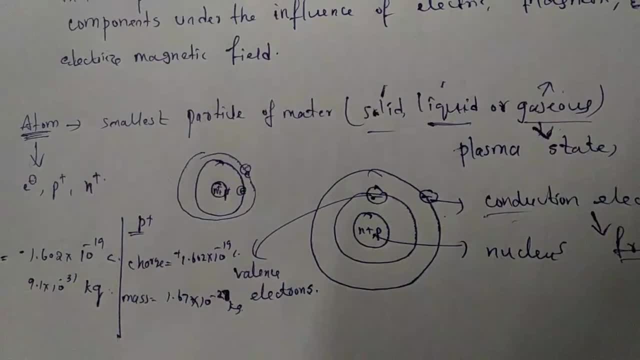 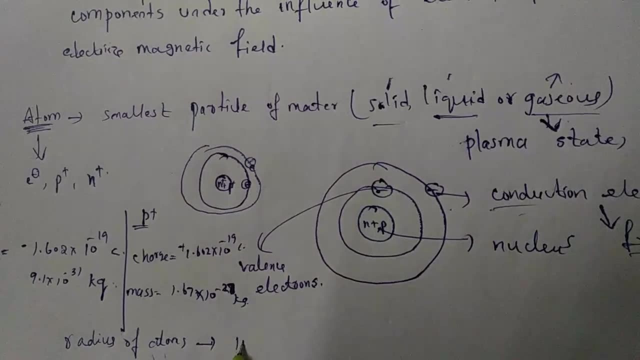 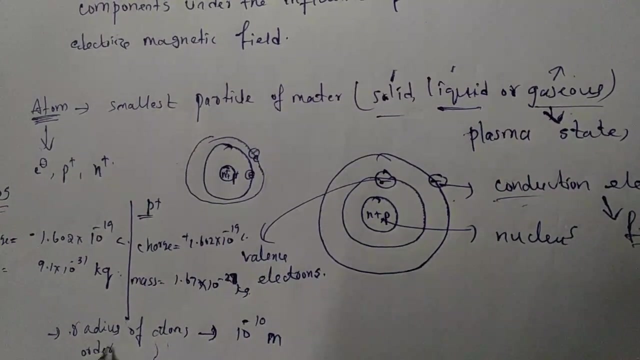 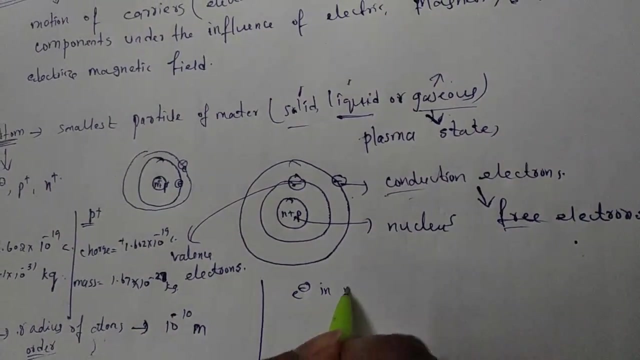 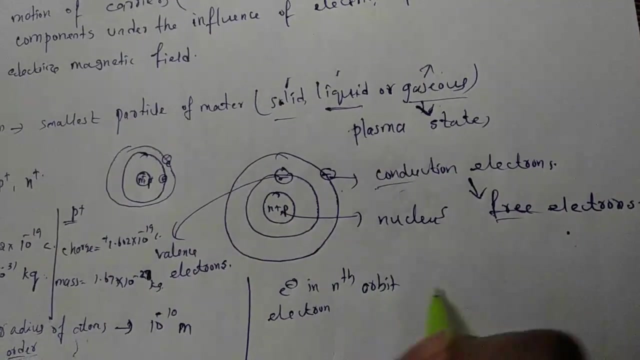 this is 27 cases. for an atom, the radius will be in the order of 10 power minus 10 meters. for autumn, this is not a value. it will be in the order of 10 power minus 10 meters. for an electron in nth orbit. electron in nth orbit has an energy. 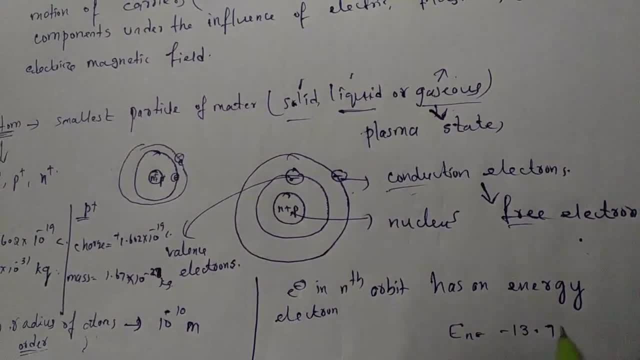 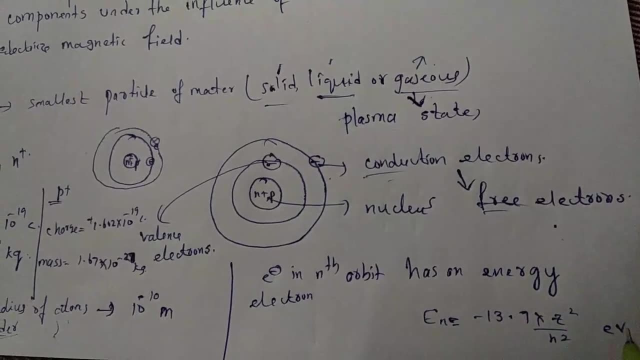 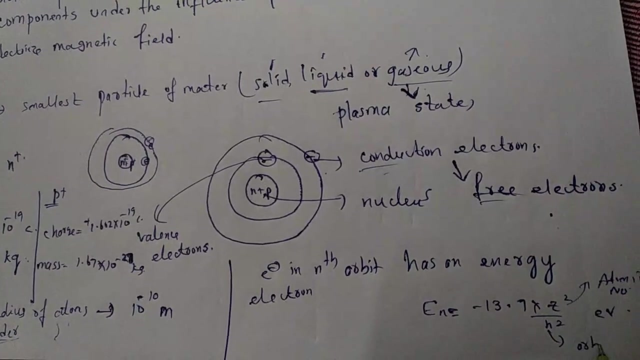 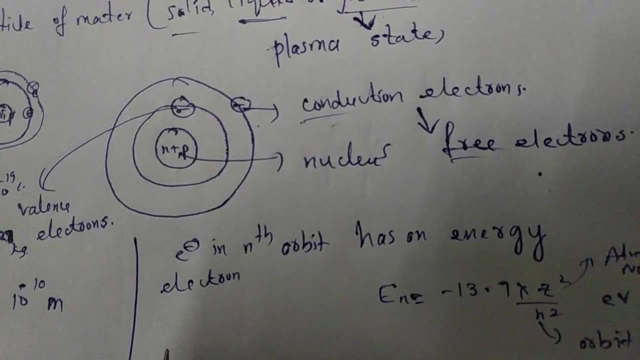 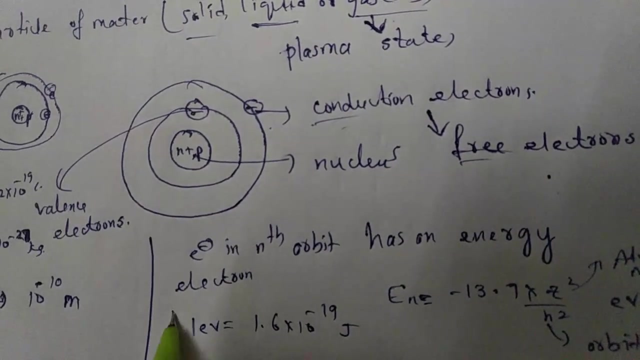 e, n, equal to minus 13.7, into z square by n square. units are electron volts. here z is atomic number and n is orbit number for conversion. 1 electron volt equal to 1.6 into 10 power minus 19 joules. now we'll see about the band diagrams. 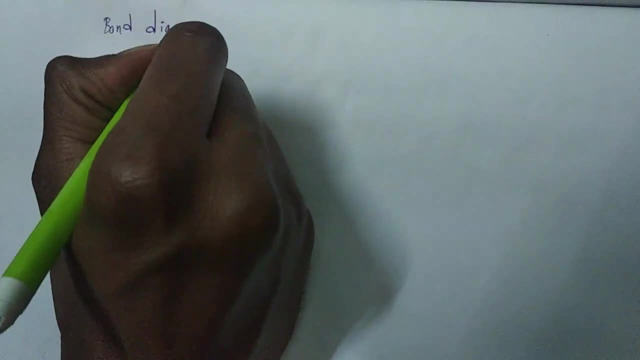 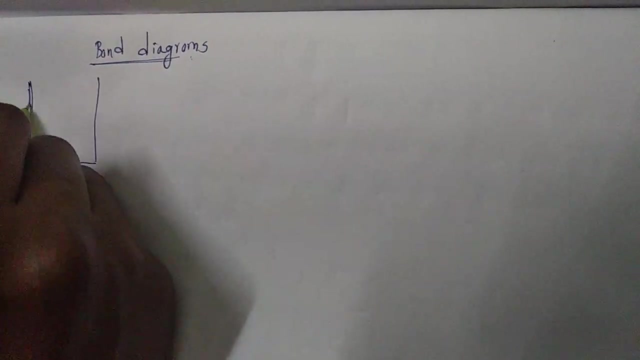 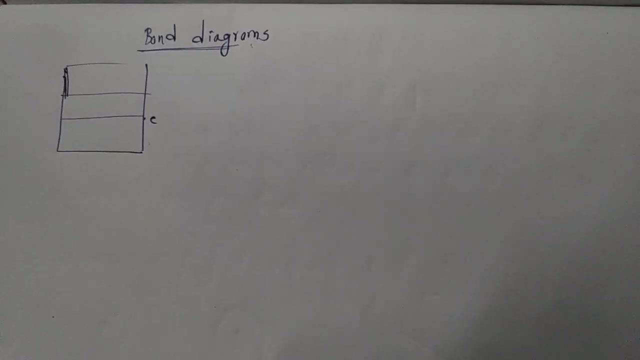 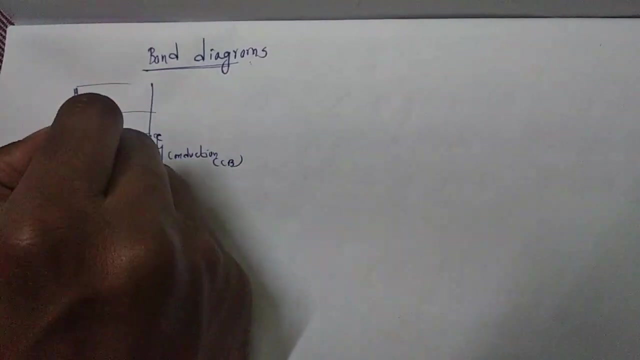 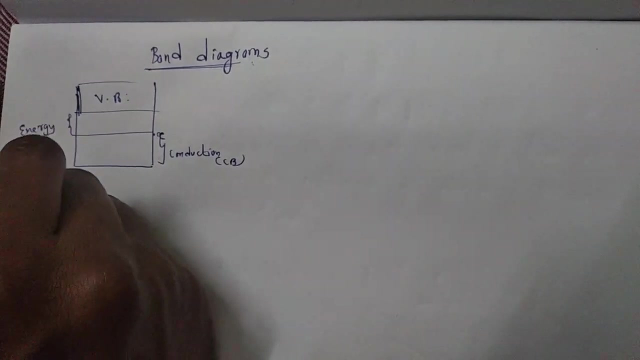 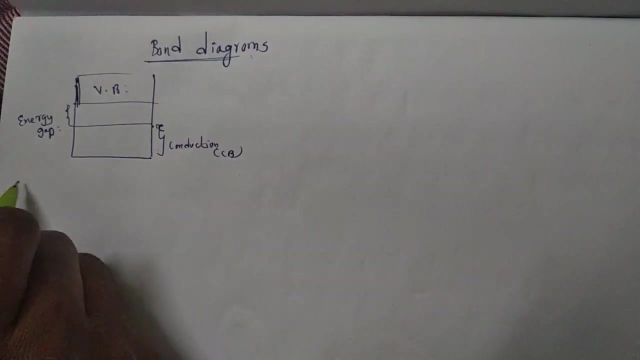 this is the energy band diagram, this is the conduction band, this is the valency band and this is the energy gap. now we'll see these three: conduction band, valency band and energy gap. first of all, we'll see the conduction band. conduction band is nothing but. 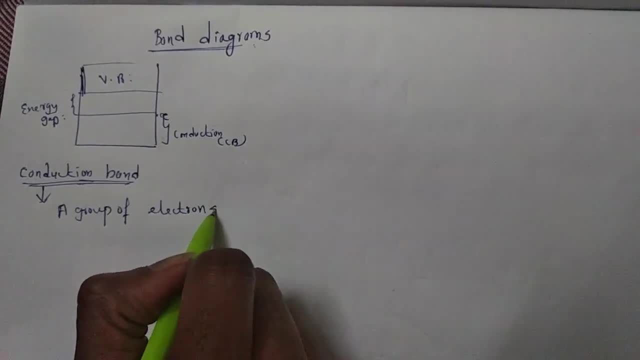 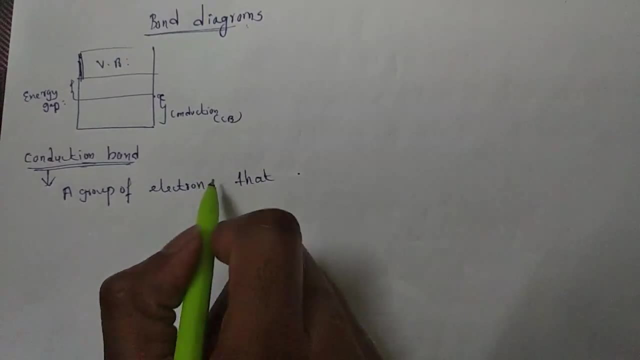 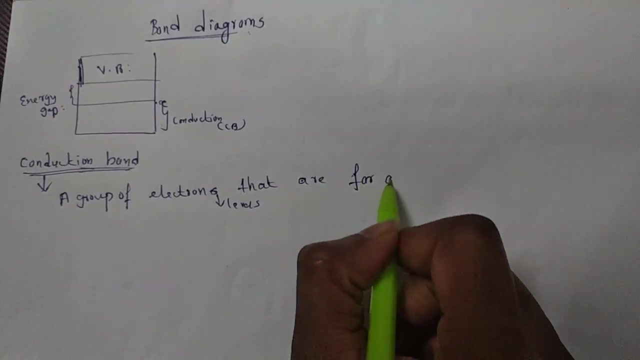 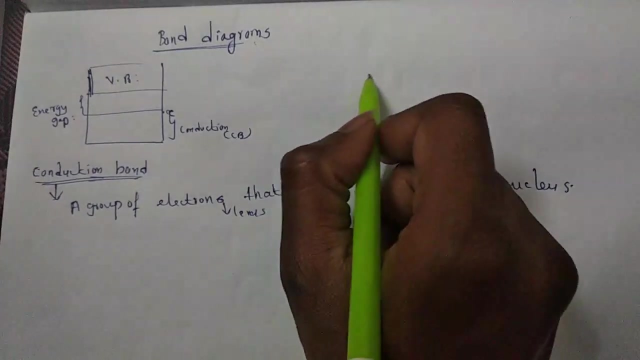 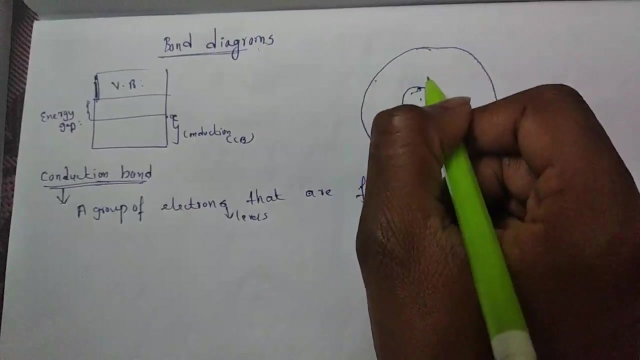 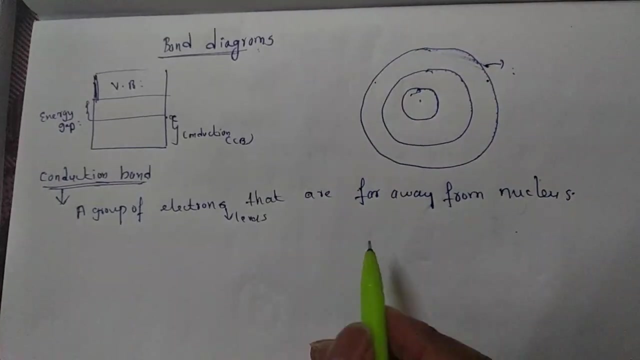 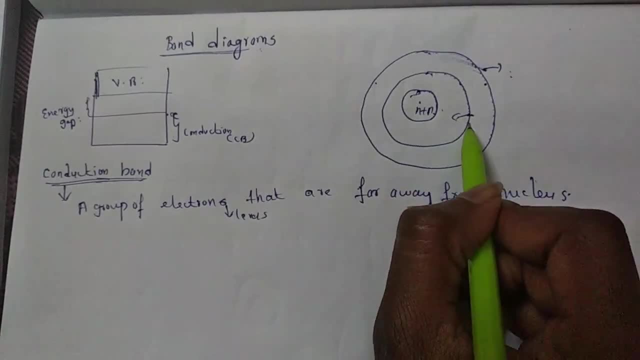 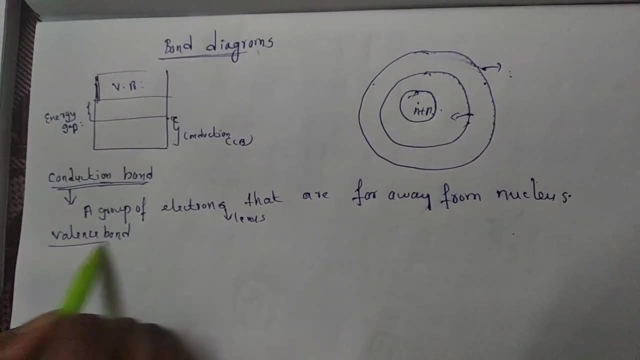 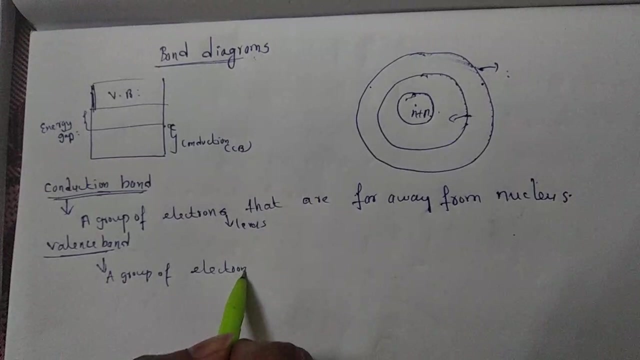 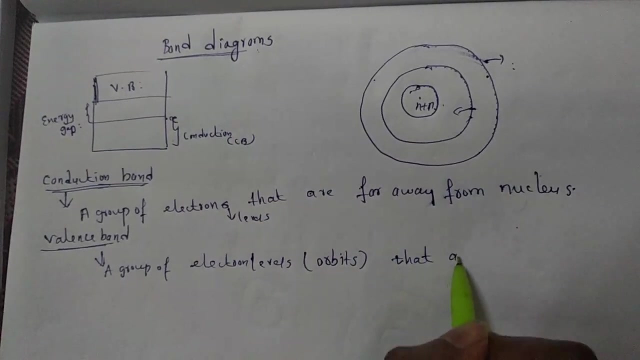 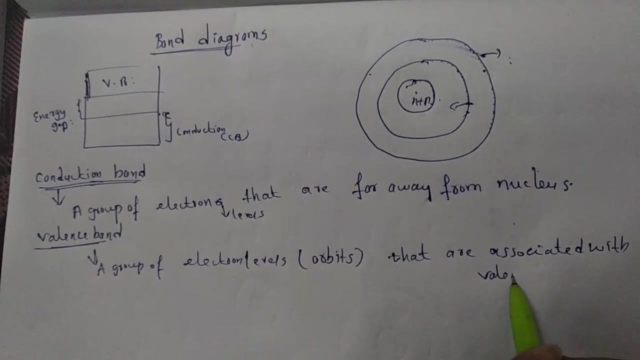 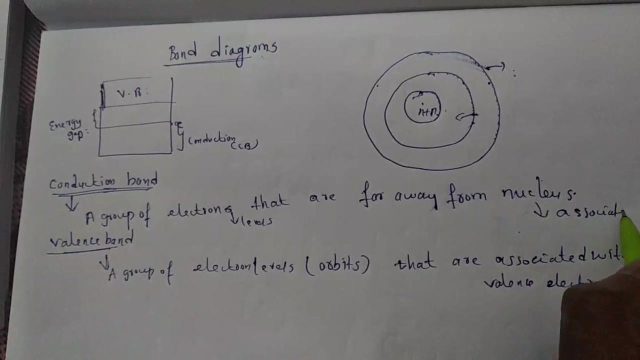 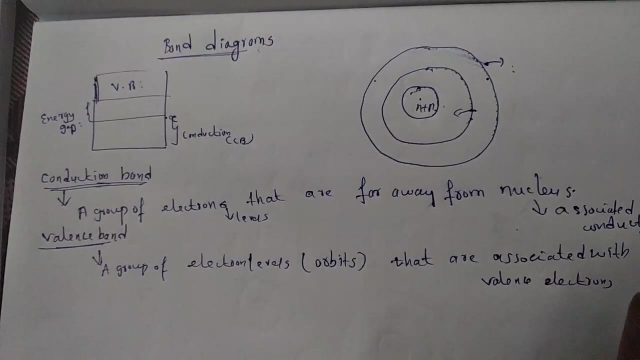 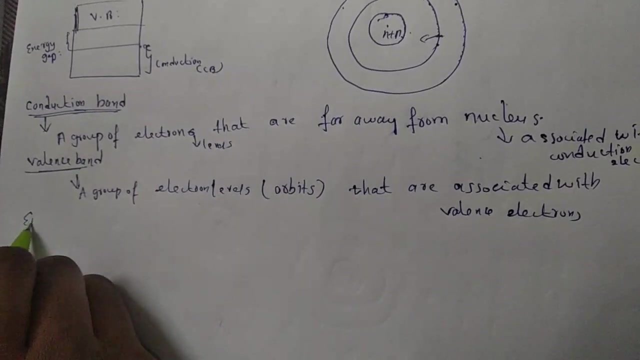 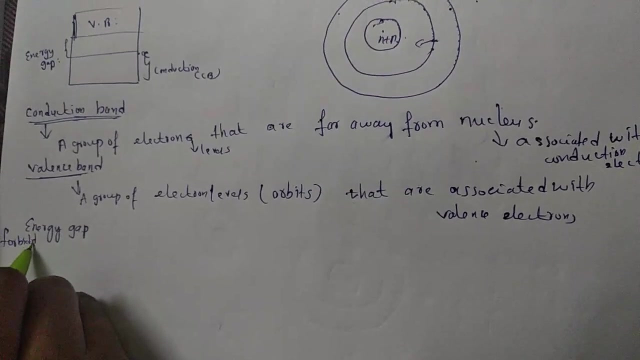 orbit. this orbit is near to the nucleus. these are known as valence band, a group of electron levels, or in another way you can say it as orbits that are associated with valence electrons, and the conduction band is associated with conduction electrons, and now we'll see the energy gap. this is forbidden energy gap. it is nothing but the. 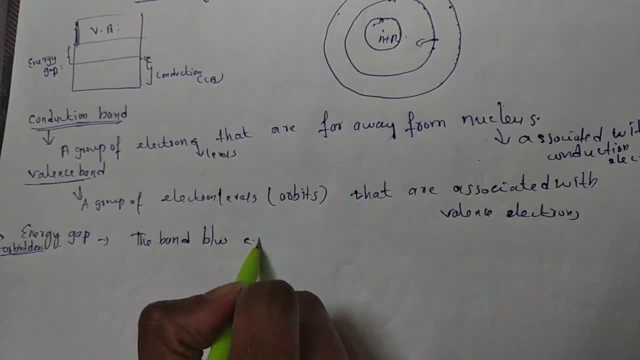 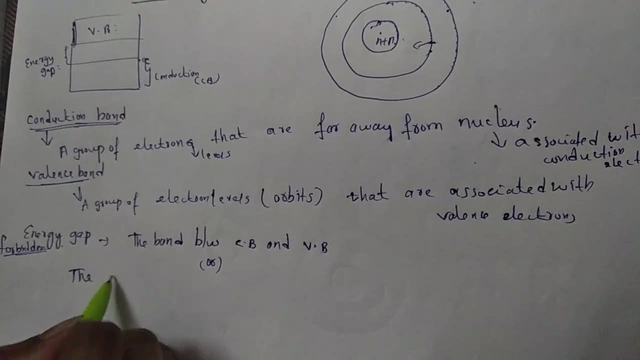 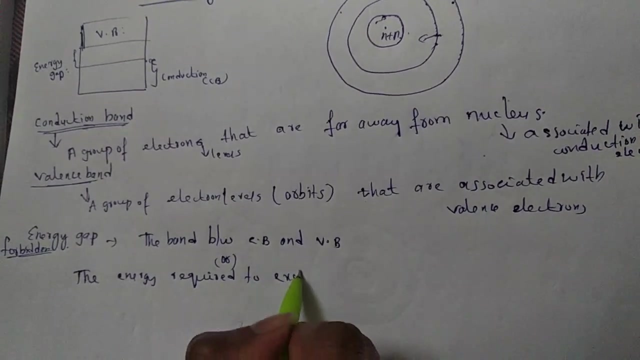 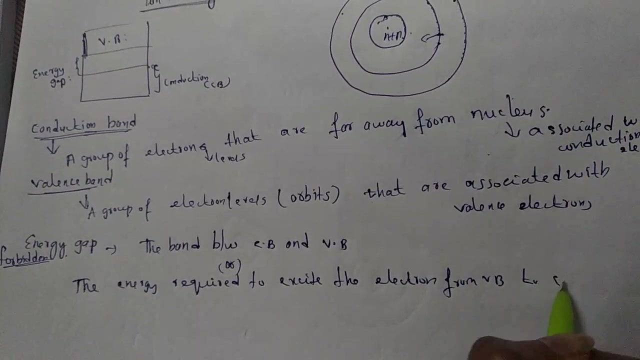 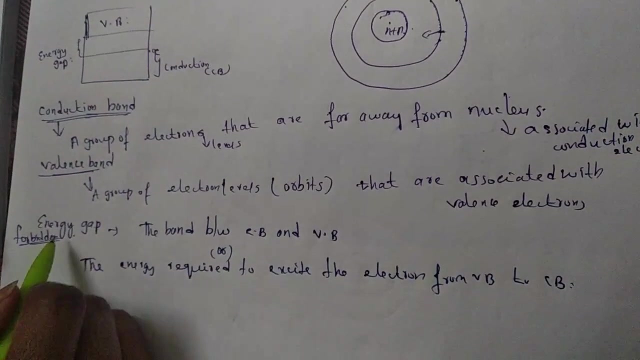 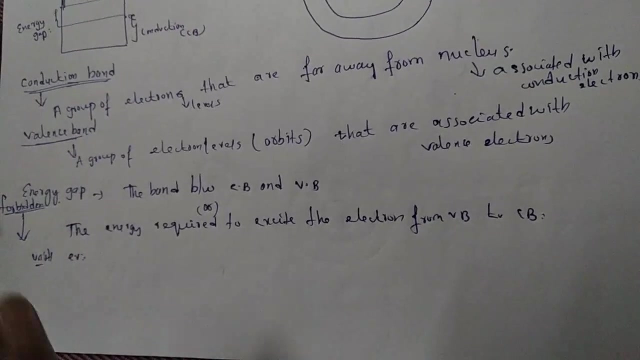 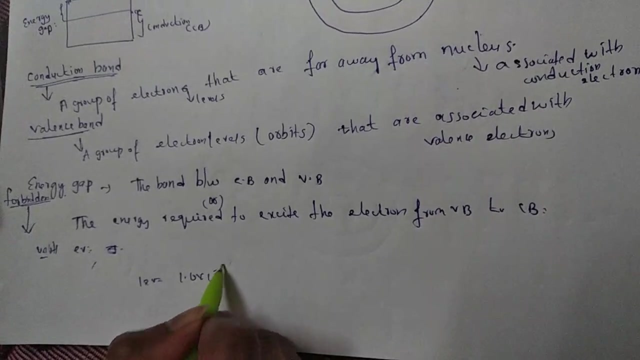 band between conduction band and valence band or, in another way, the energy required to excite the electrons from valence band to conduction band. this is known as 4 billion energy gap and this connection, this energy gap units are electron volts. this units may be in terms of joules also: 1eV equal to 1.6 x 10-19 joules. 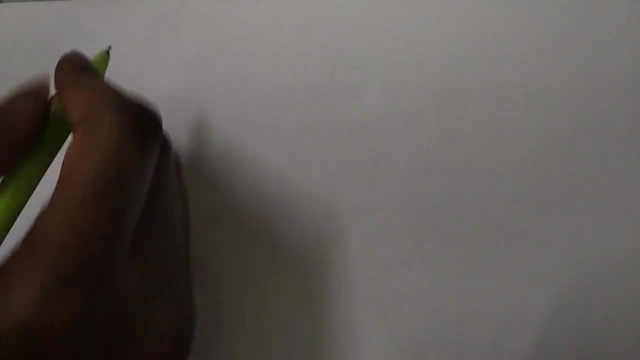 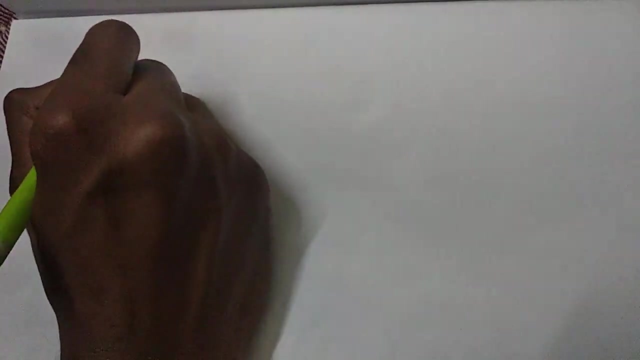 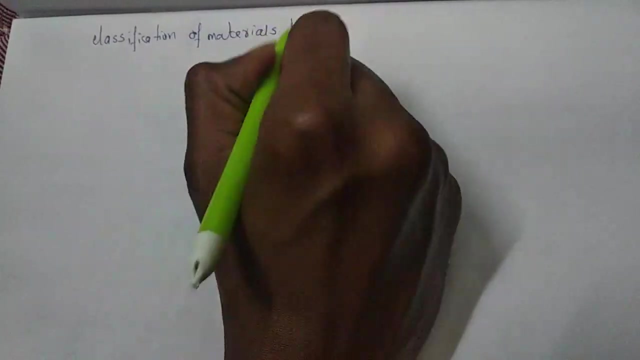 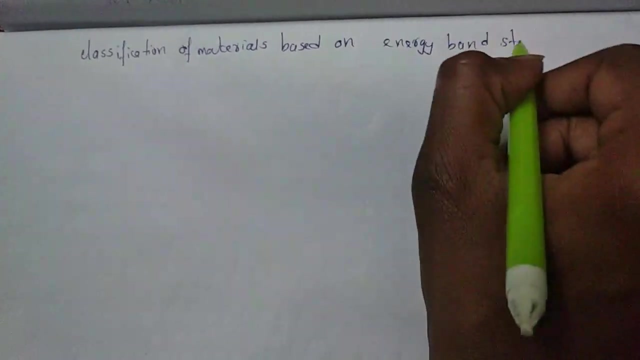 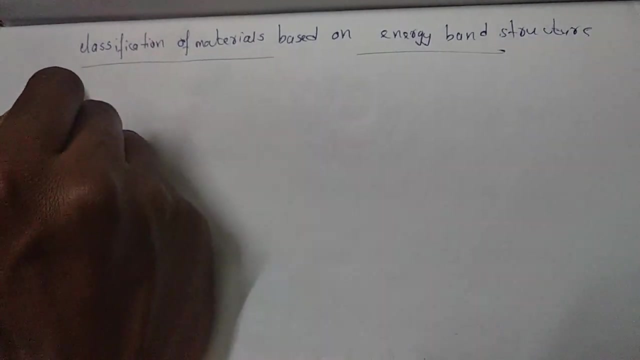 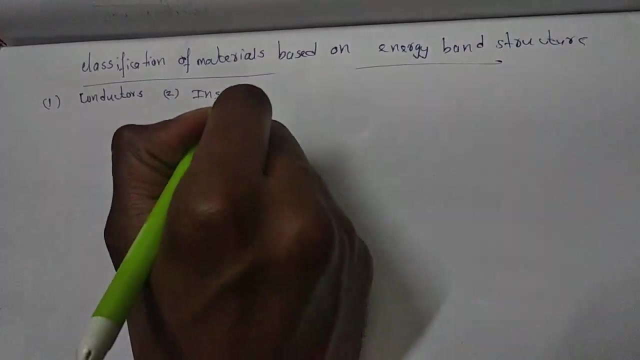 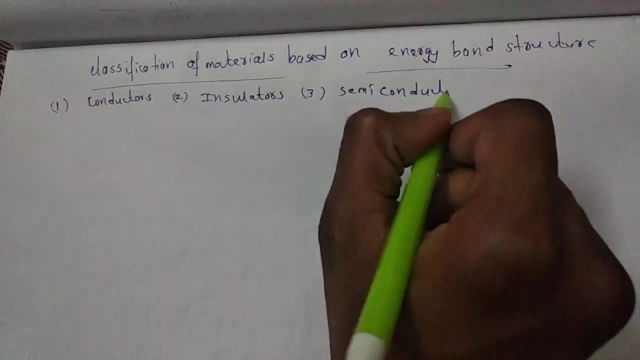 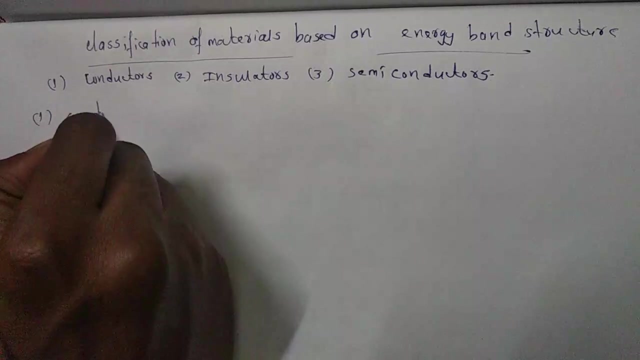 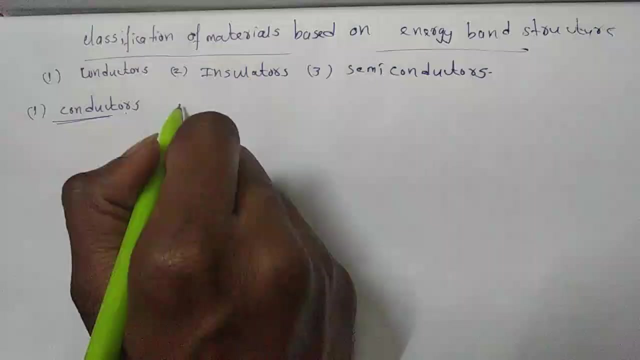 now we will see the classification of materials based on energy band gaps, based on energy bank structure. there are three types of materials: first one conductors, second one insulators and the other half semiconductors. first of all, we will discuss about conductors. now let us consider the band diagram. 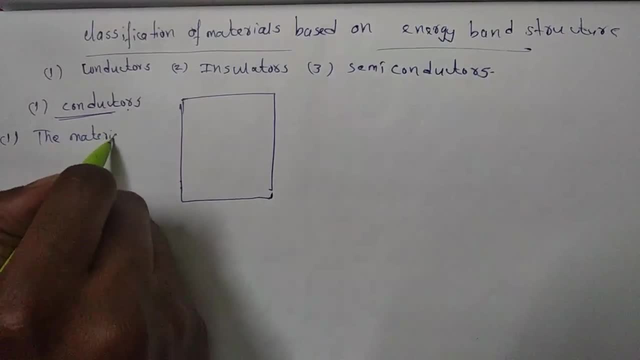 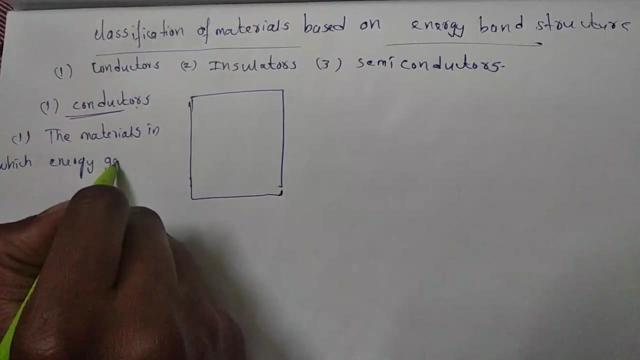 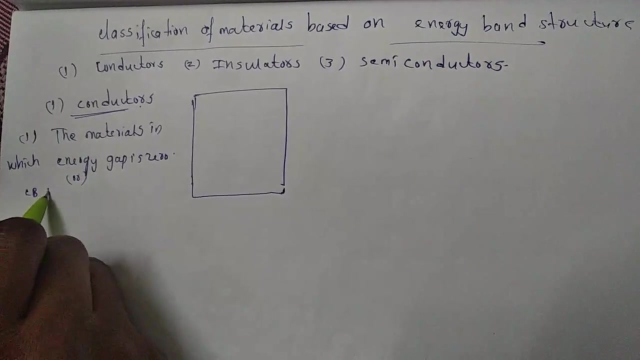 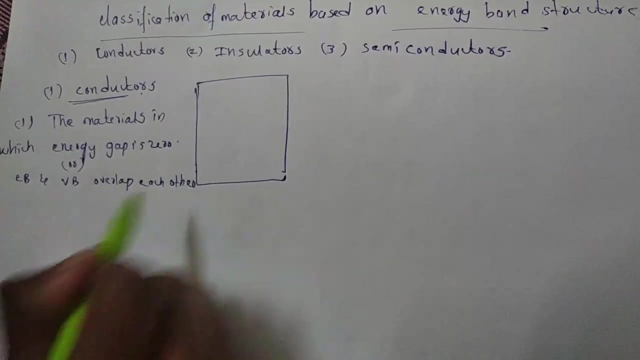 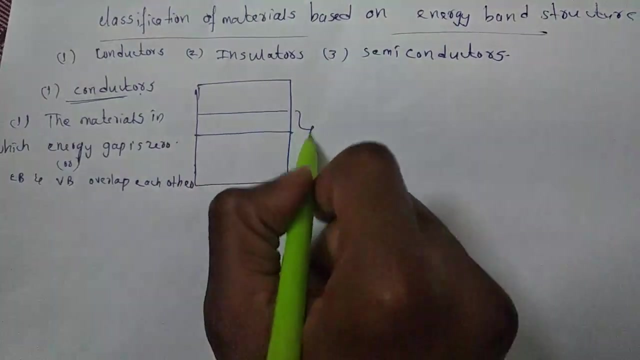 CFG, in which energy band gap is zero, or in another way we can say it, as the conduction band and valency band overlap each other. up to this, this is the valency band and up to this, this is conduction band. here we can see that if 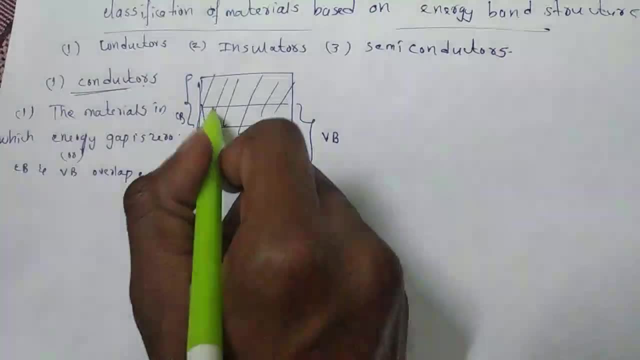 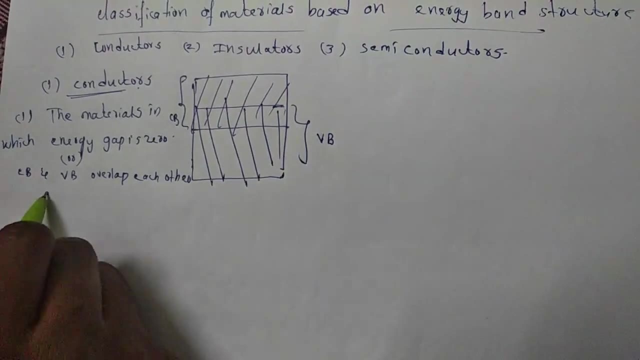 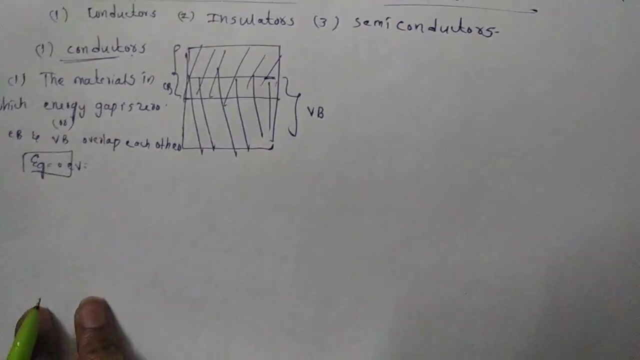 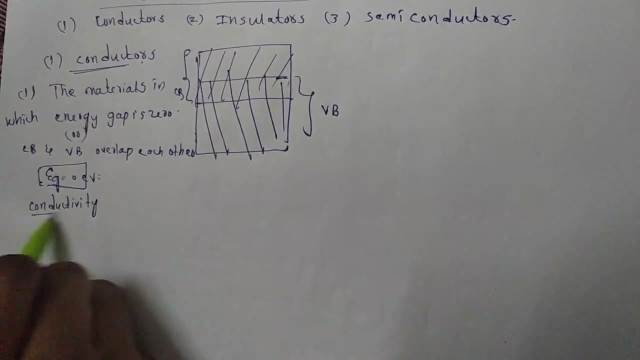 you take, this is as conduction band and this is as valency band. these two are overlapped each other. that means there is no energy gap. the energy gap is zero electron volts. these are the conductors. now coming to its property, we will discuss conductivity. conductivity is: 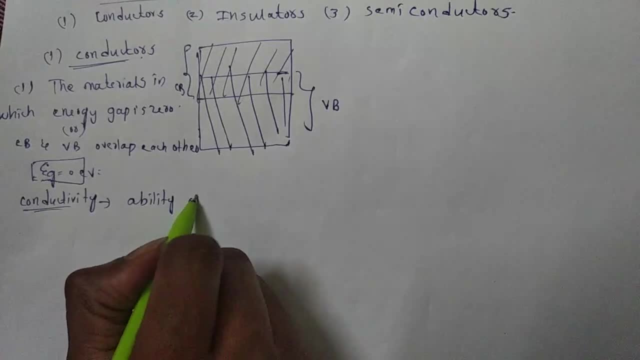 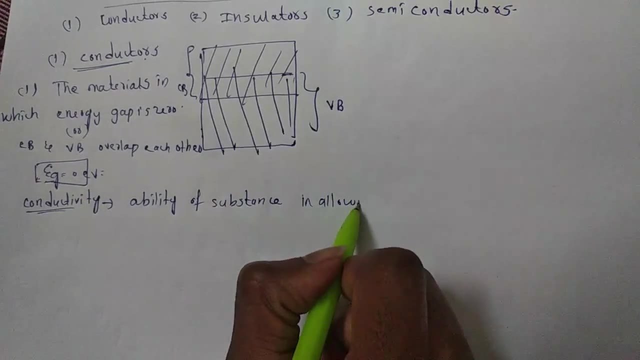 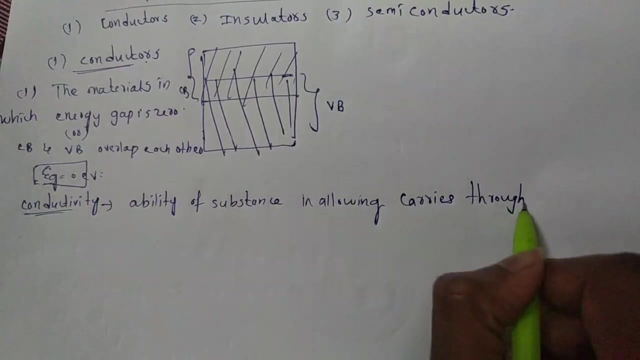 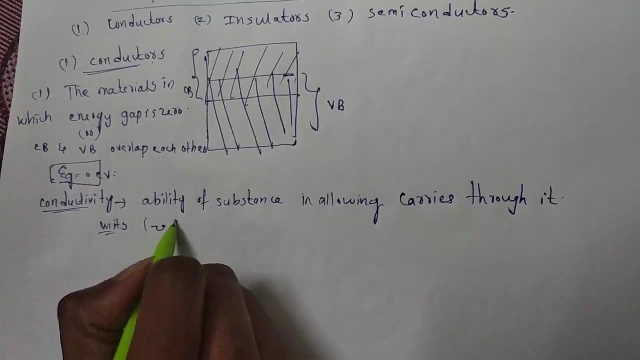 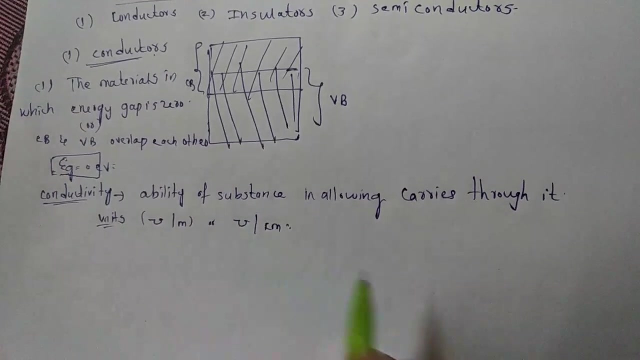 nothing but the ability of material or substance. so it is magnetic and it will have a magneticKY degree despite its conductivity, its resistance, the relative. we will talk on that in the next final class that today we can take itsocracy through. here we have a Michigan current. 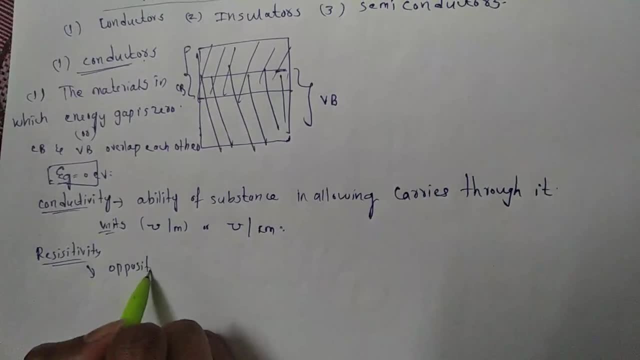 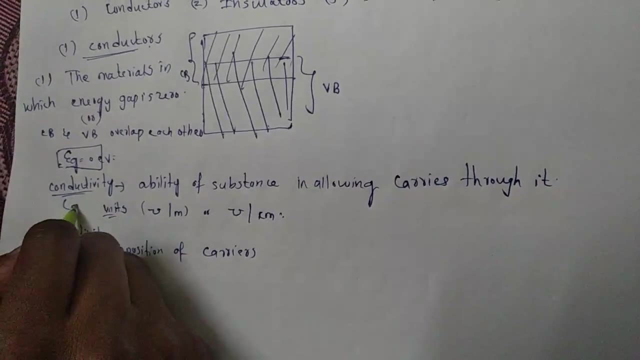 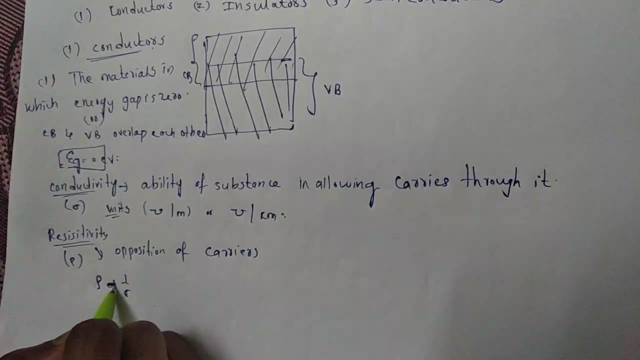 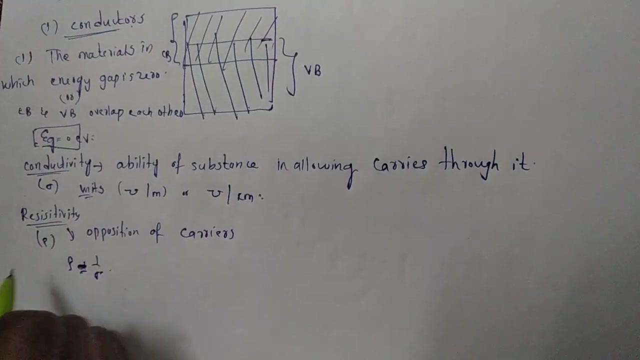 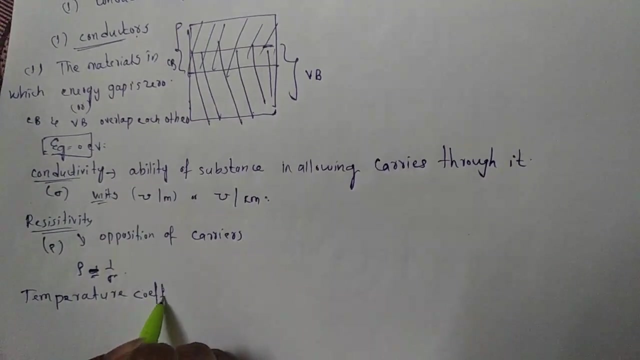 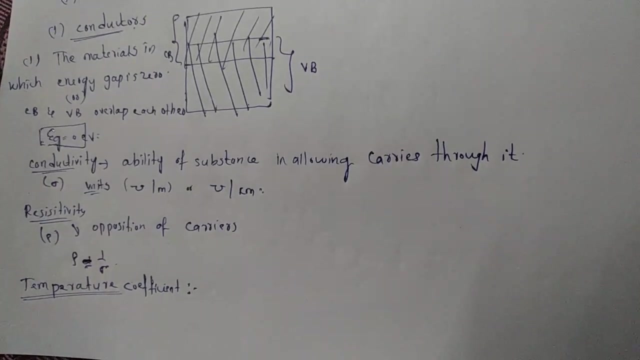 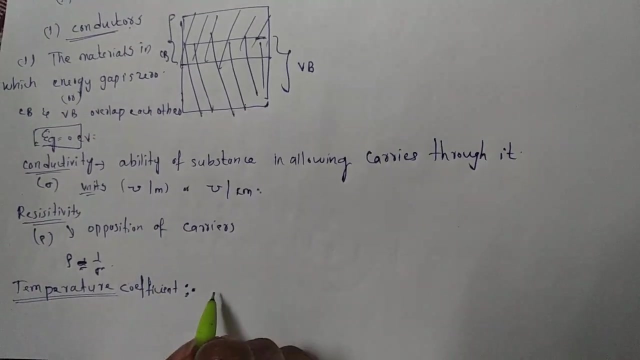 cooperation, fish industry and how to opposing of carriers. just inverse of the conductivity is resistivity. the resistivity and this conductivity are inversely proportional, or simply this resistivity equal to 1 by Sigma. we will see another property called temperature coefficient. the is very important property while making of any materials temperature coefficient means. 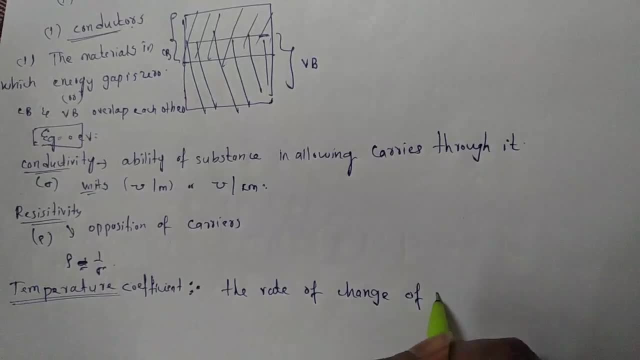 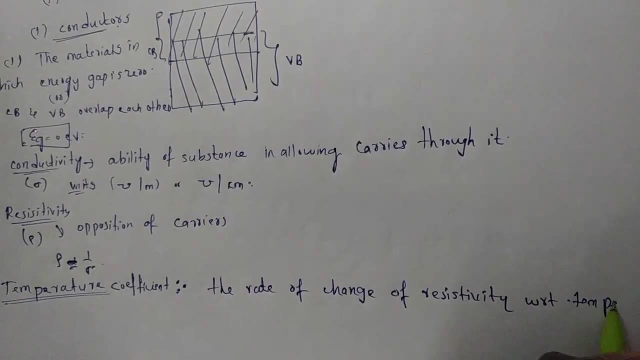 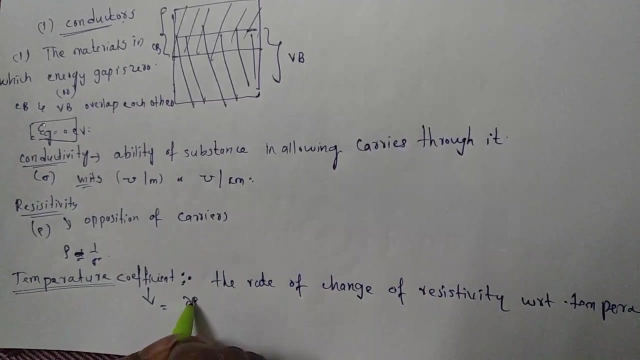 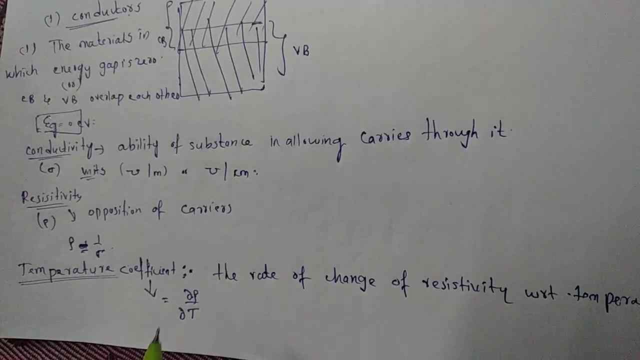 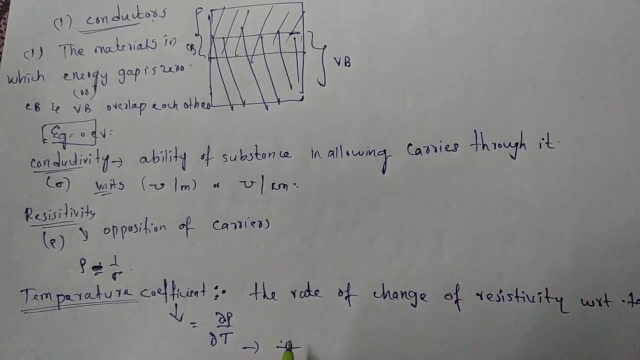 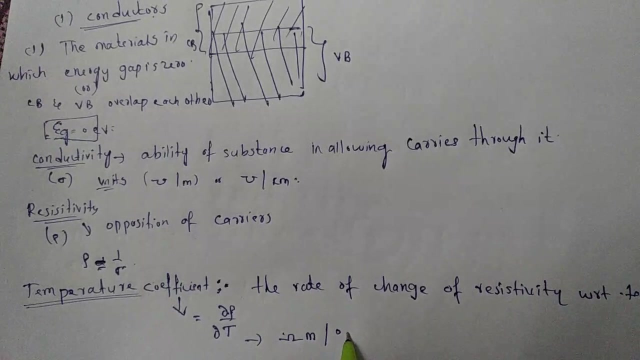 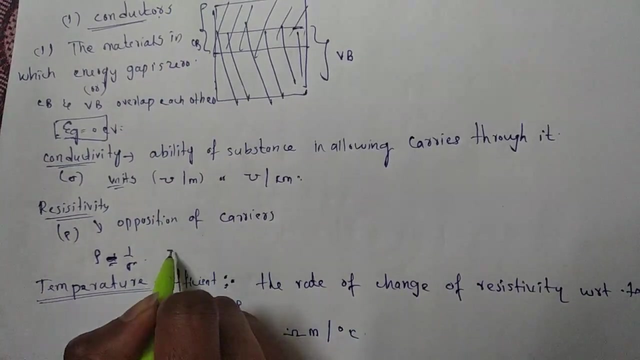 the rate of change of resistivity with respective to temperature. this temperature coefficient equal to this is rate of change of h2b. that means dou rho by dou t. this temperature coefficient units are ohm meter per degree centigrade and this is alpha. here the resistance units are ohm meter. here see the units, the coefficient. 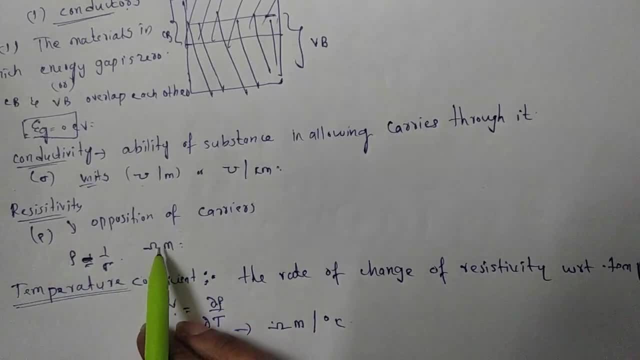 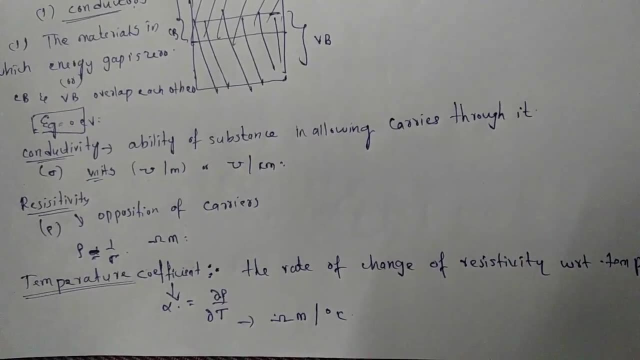 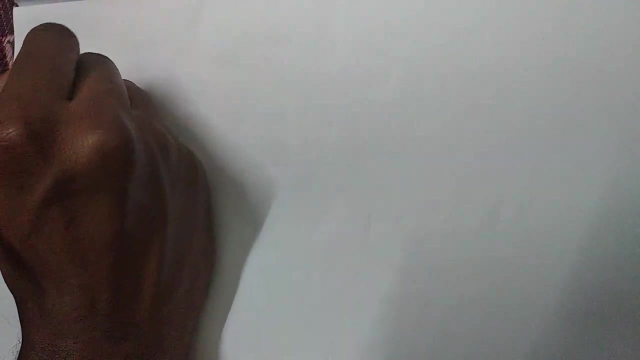 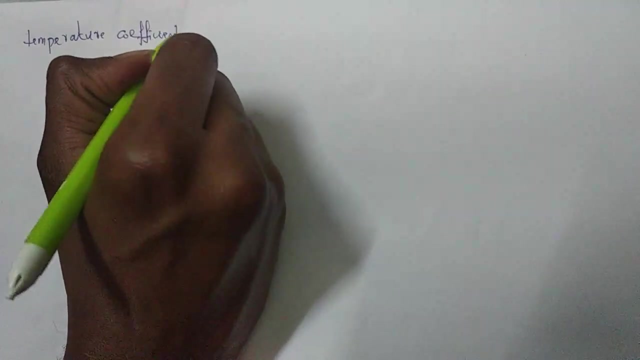 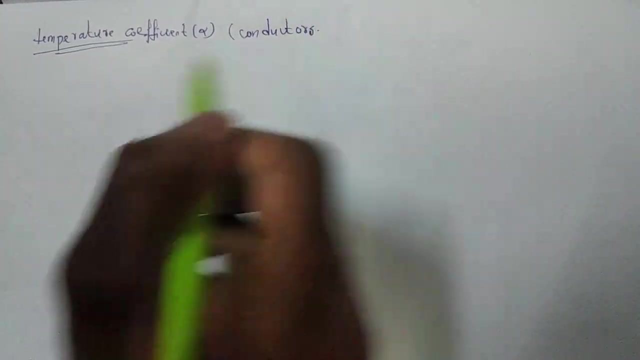 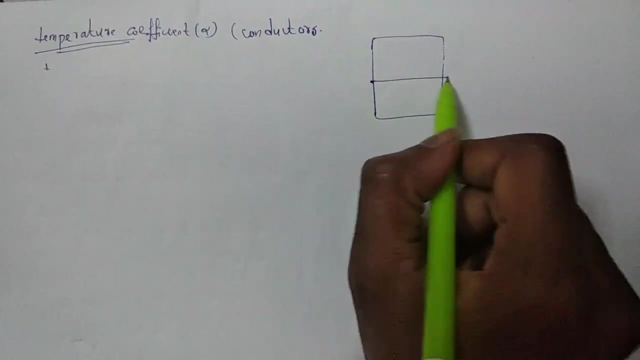 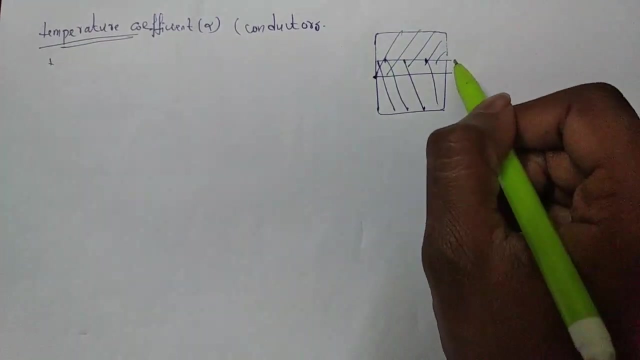 of conductor units are: mo per meter. resistivity, ohm meter. temperature coefficient. ohm meter per degree kelvin. now we will see how the temperature coefficient for conductors. now we will see how the temperature coefficient for conductors, for conductors, for conductors. let us consider the band diagram for conductors. 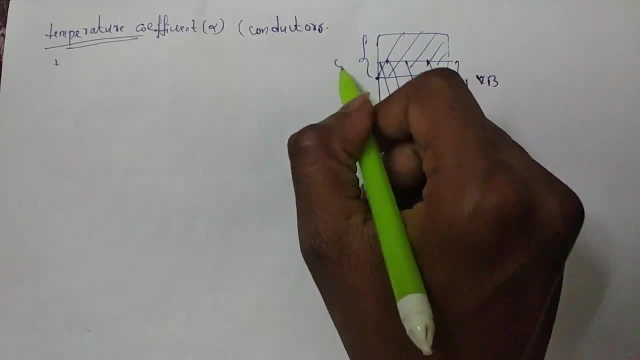 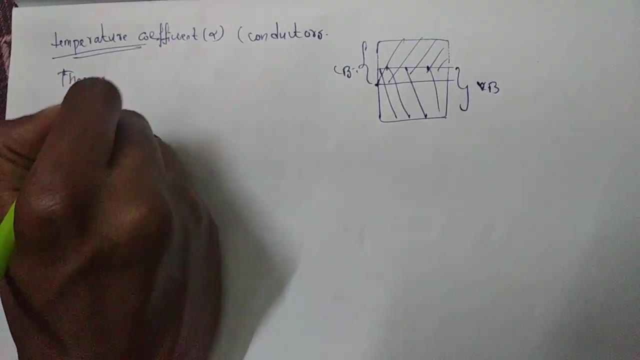 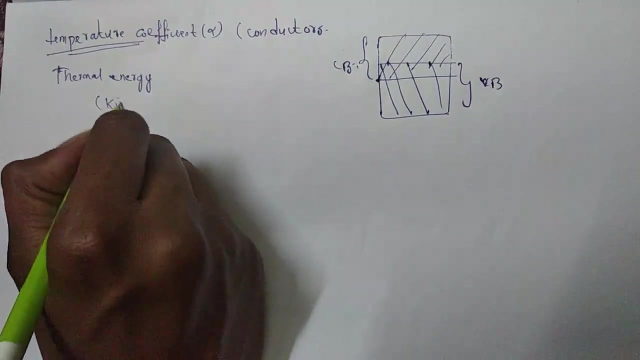 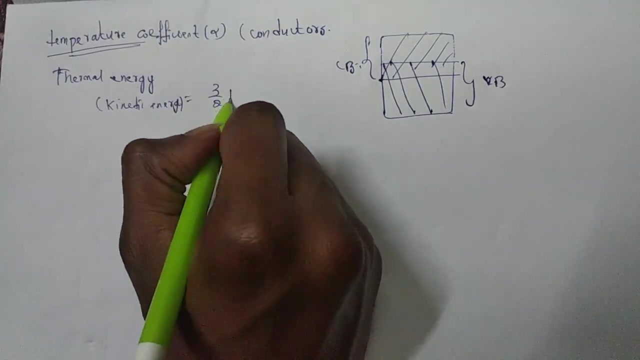 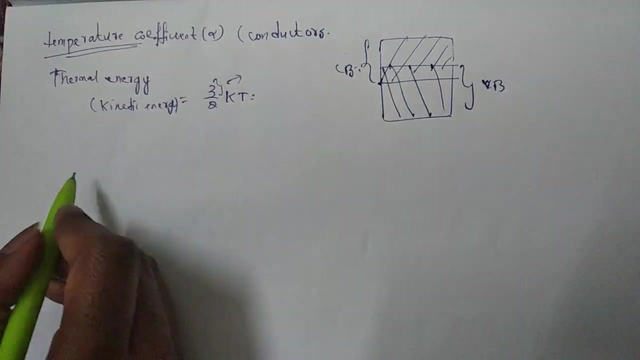 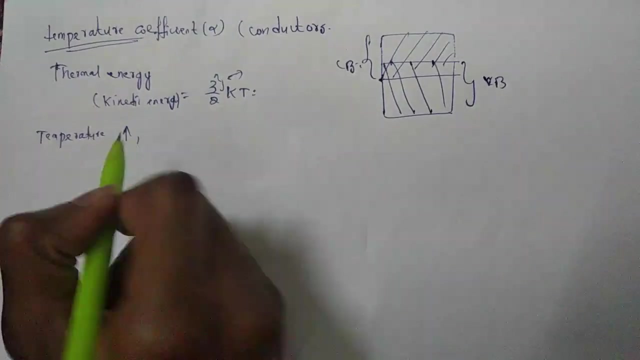 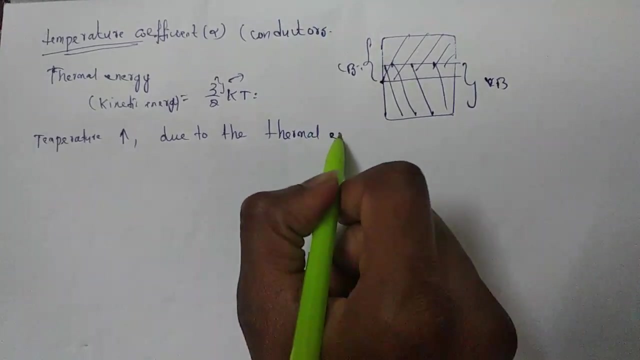 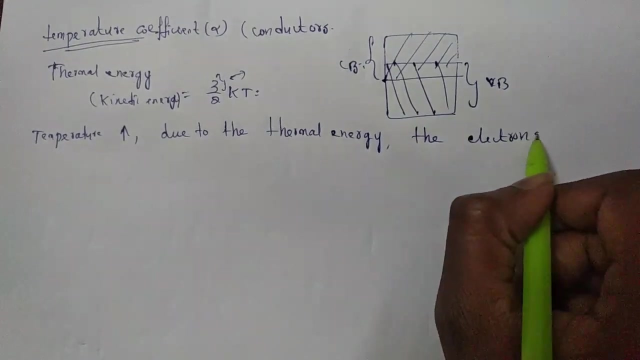 this is conduction, this is valence band and this is conduction band. we know that thermal or the kinetic energy equal to 3 by 2 into kT. here the value will be changed based on the decrease of freedom as the temperature increases due to the thermal energy, the electrons. 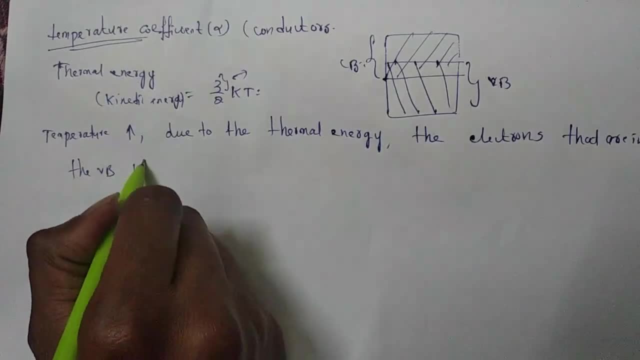 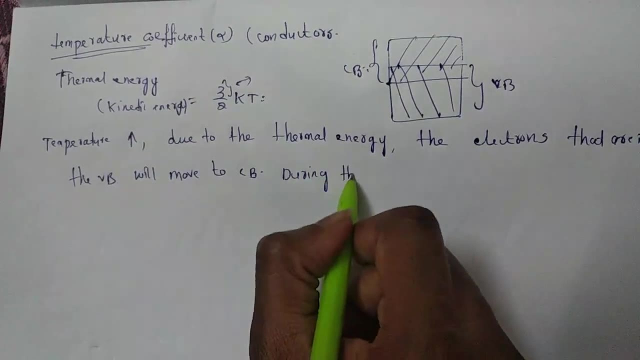 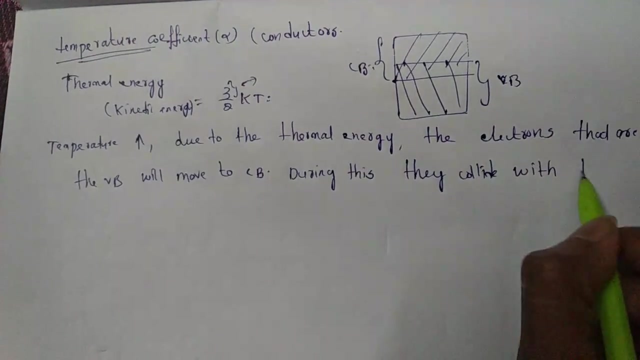 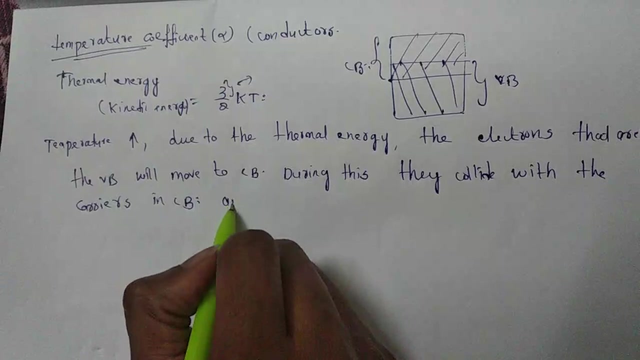 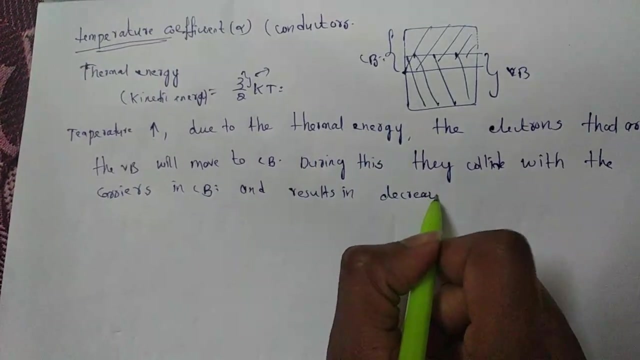 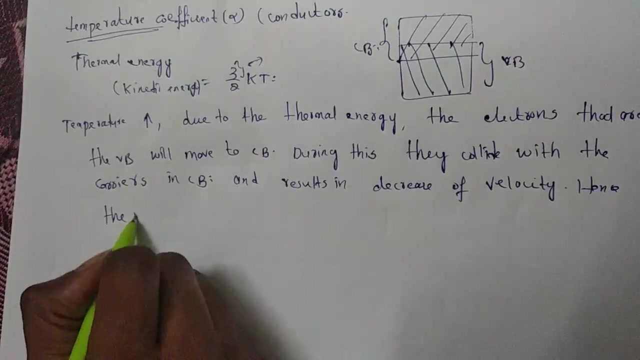 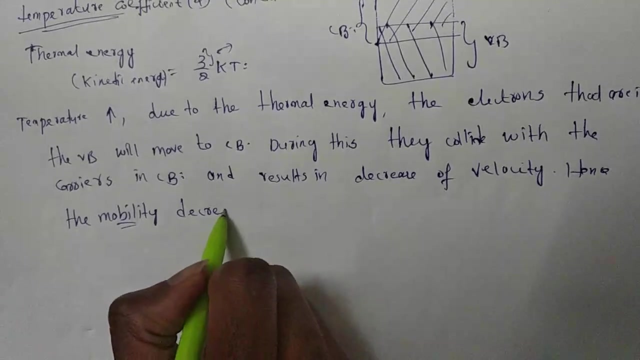 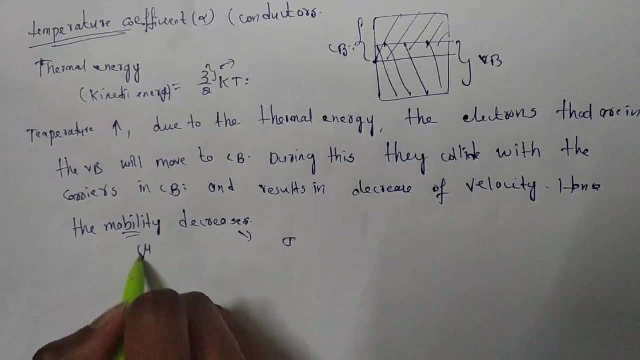 that are in the valence band will move to conduction band. during this they collide with the carriers in conduction band and results in decrease of velocity. Hence the mobility decreases. Mobility means nothing but a movement, nothing but velocity. As the mobility decreases- this is mu- the conductivity increases. This conductivity. 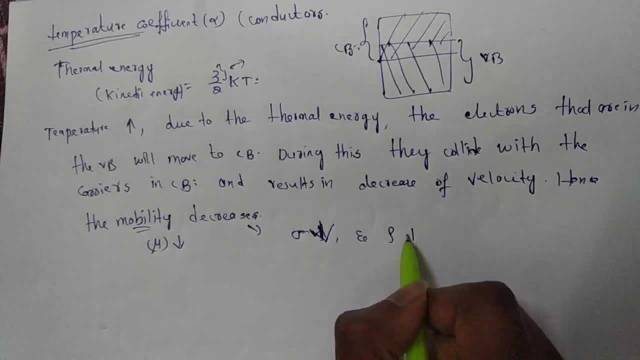 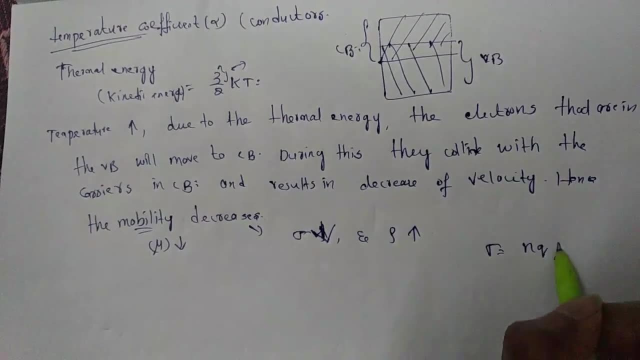 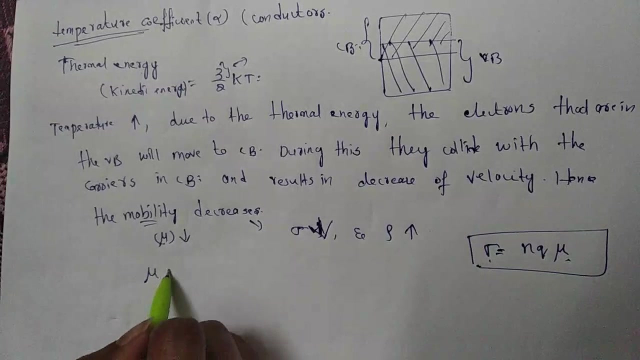 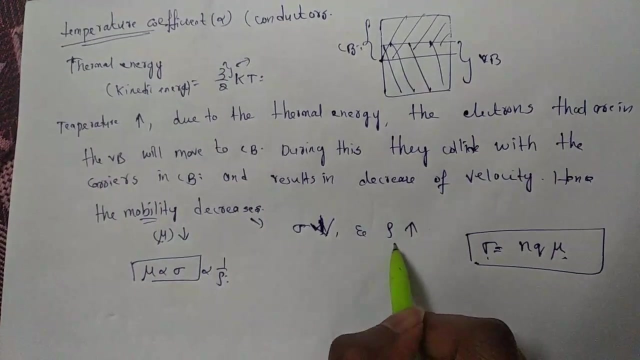 decreases and the resistivity increases. Here we will see one equation: This conductivity equal to n, into q, into mu. We will see this in later videos. Sigma and mu are directly proportional And this is inversely proportional to drop As the temperature is increasing. 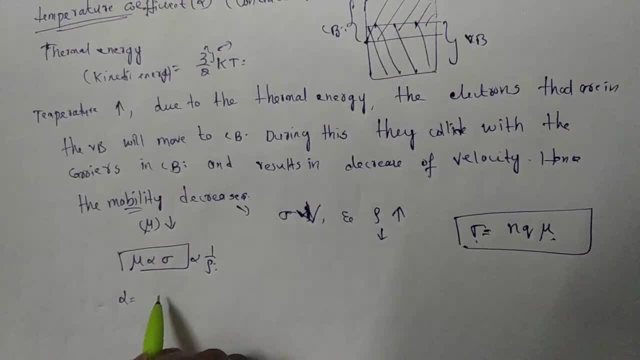 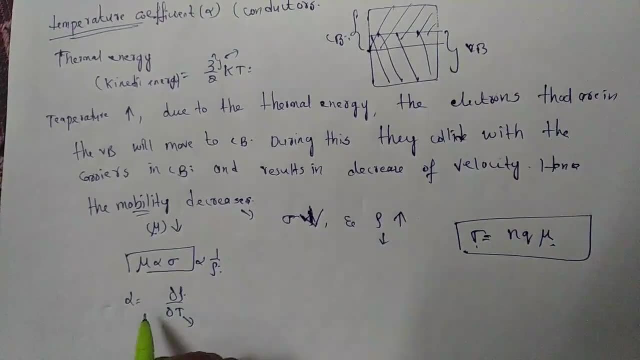 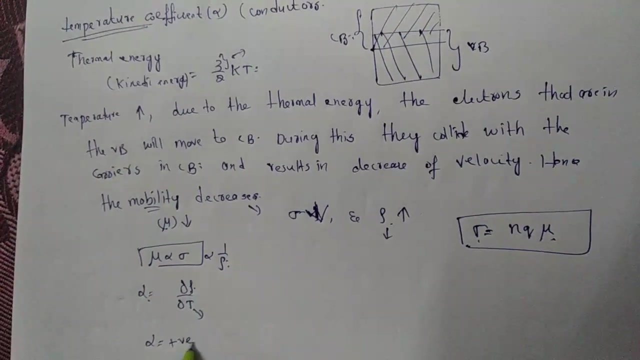 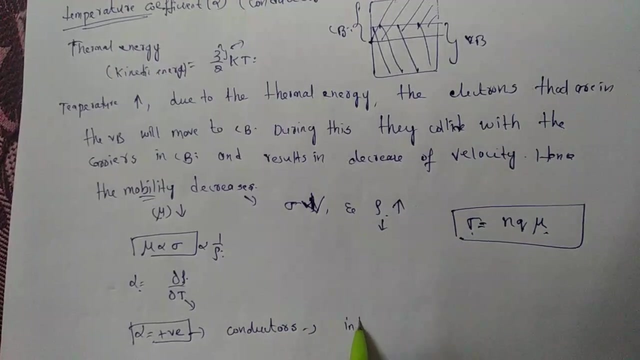 the resistivity is increasing. You know that temperature coefficient alpha equal to dou rho by dou t. As the temperature is increasing, the rho value is decreasing, The rho value is also increasing, Hence the alpha will be positive for conductors. This is for intrinsic 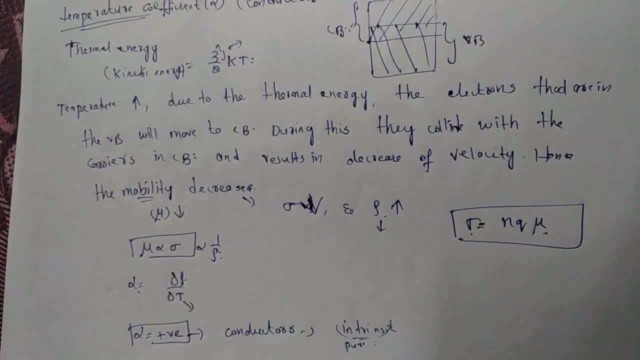 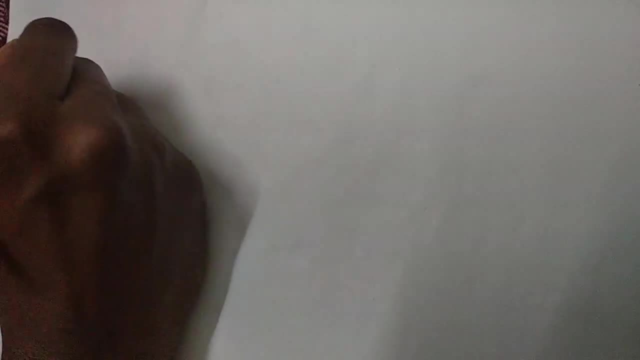 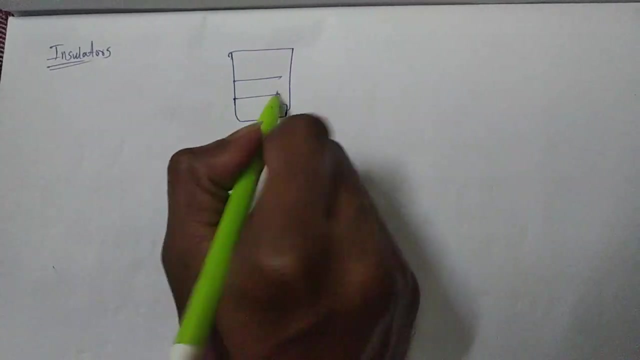 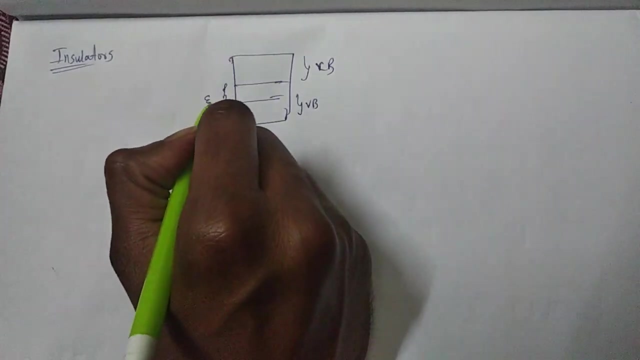 pure. We will discuss this later. Meanwhile, it will remain that alpha is positive for conductors. Now we will see about insulators. Consider the band diagram. This is conduction band and this is valence band. This is forbidden energy band. EG Insulators are nothing but. 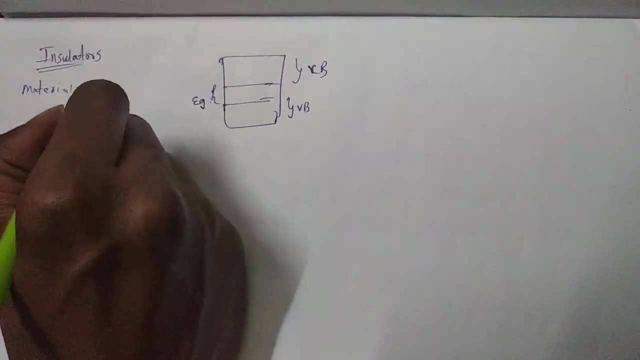 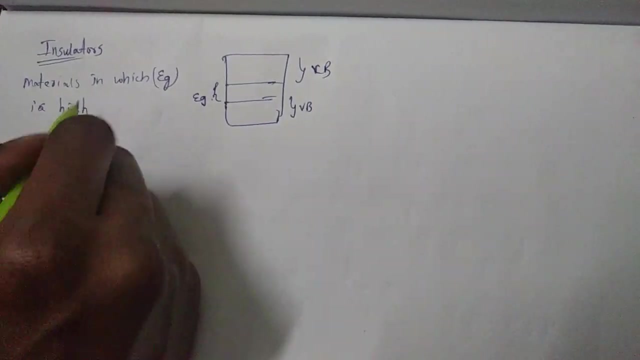 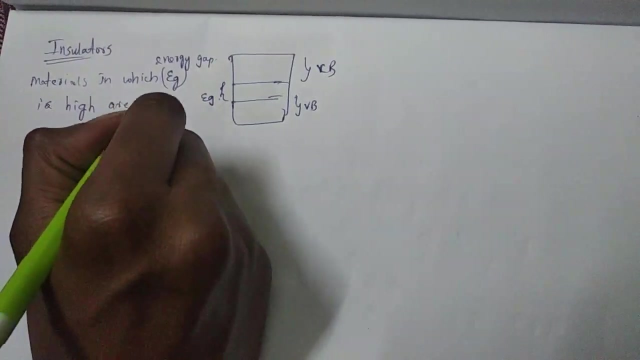 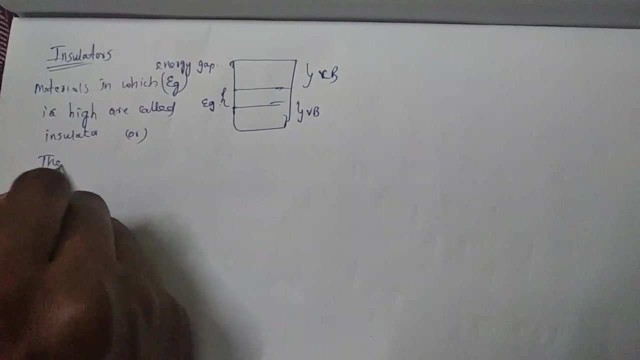 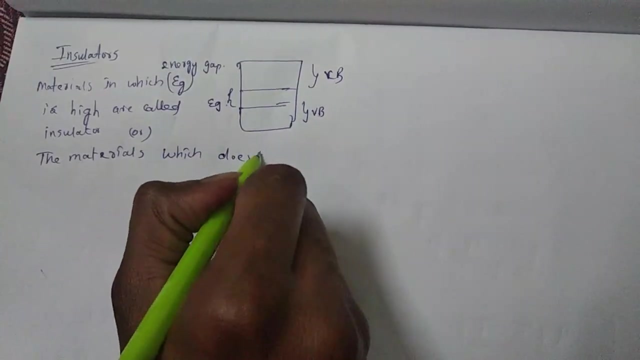 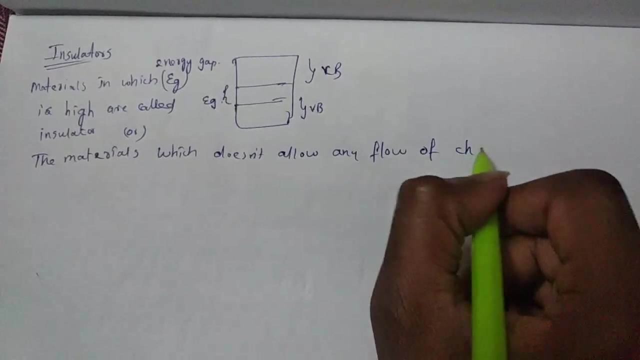 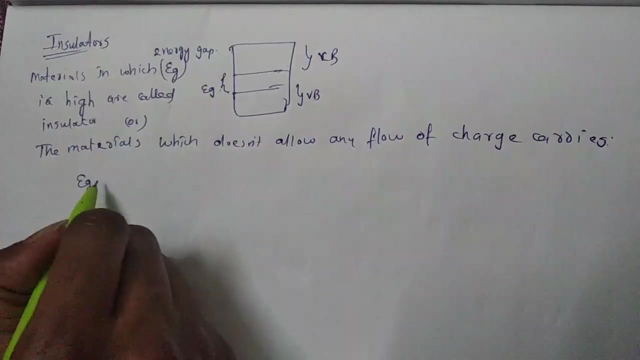 the materials in which energy gap is 0. High, or call insulators, Or, in another way, the materials which doesn't allow any flow of carriers. For insulators, the energy gap of EG is greater than or equal to six electron volts. 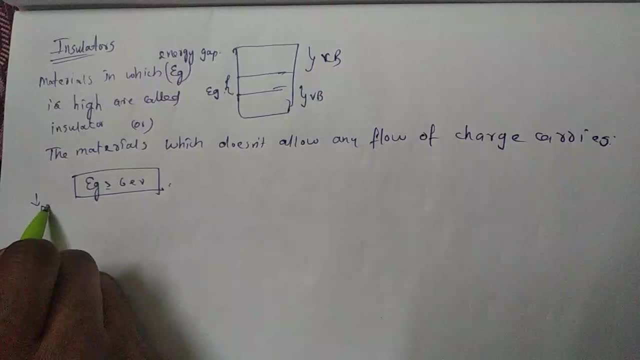 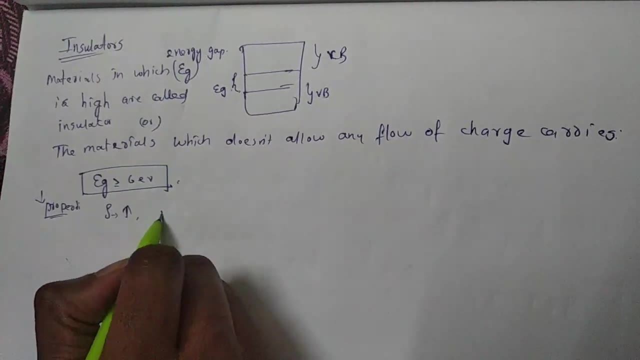 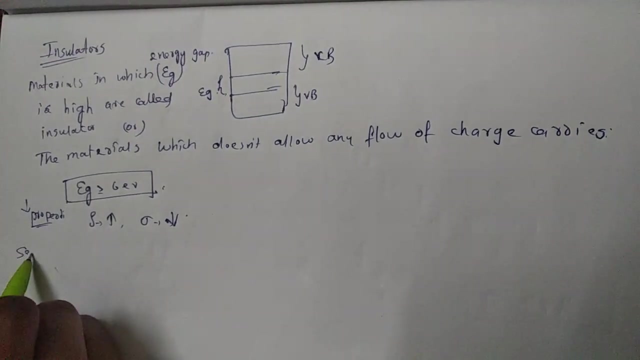 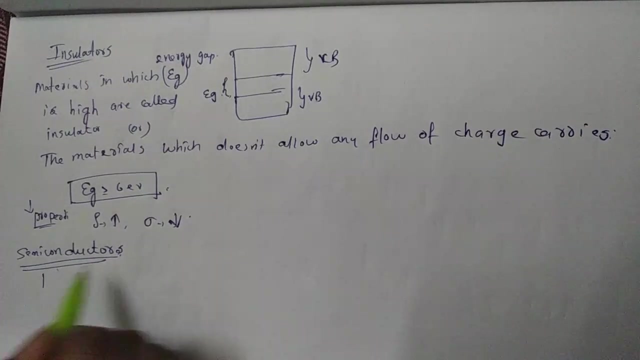 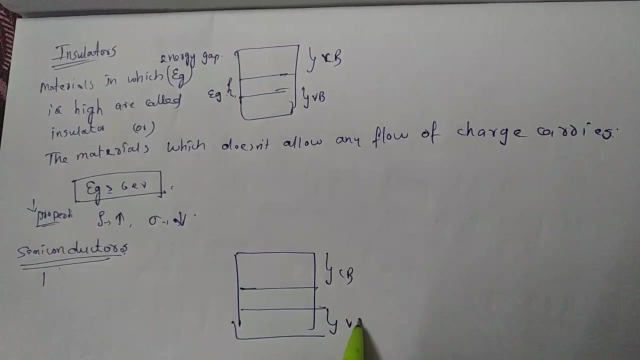 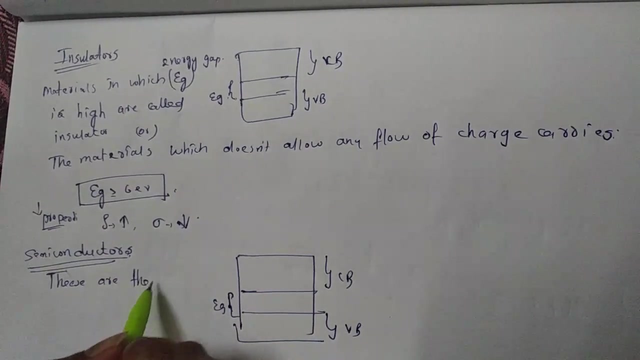 On coming to the properties, the resistivity is very high. As the resistivity is high, the candectivity will be very low. Coming to semiconductors, EG is very new. We discussed that in previous lessons There. consider the energy band diagram. this is the energy gap. these are the materials. 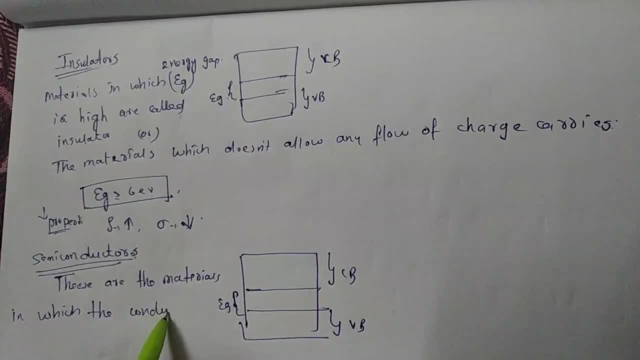 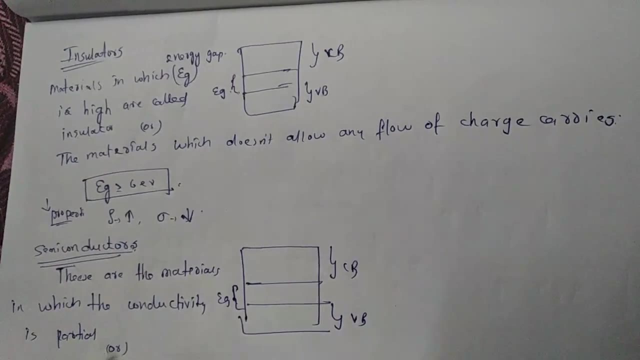 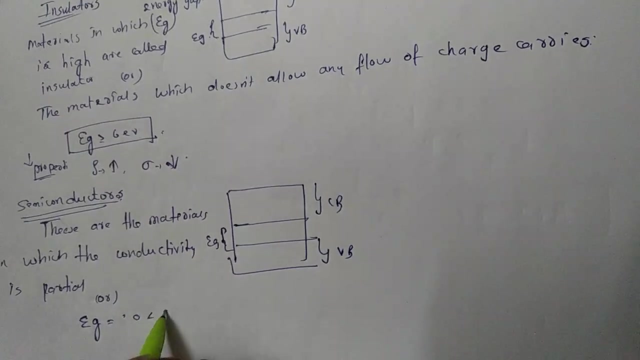 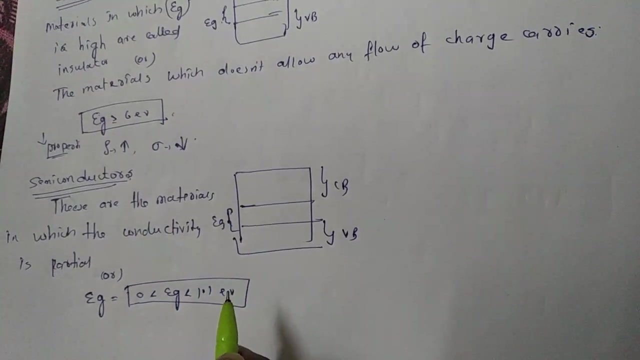 in which the conductivity is partial, or these are the materials in which the energy gap lies between 0 and 1.1 eV. when coming to these properties, the conductivity is partial, or these are the materials in which the energy gap lies between 0 and 1.1 eV.